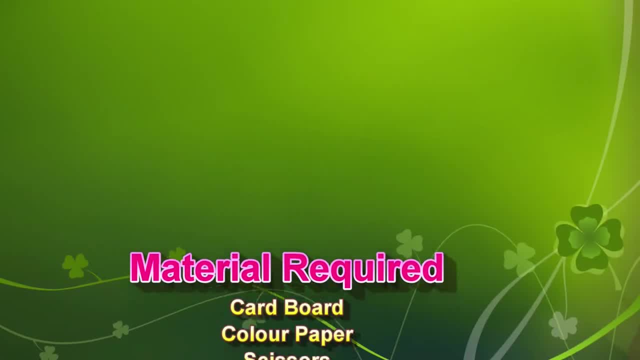 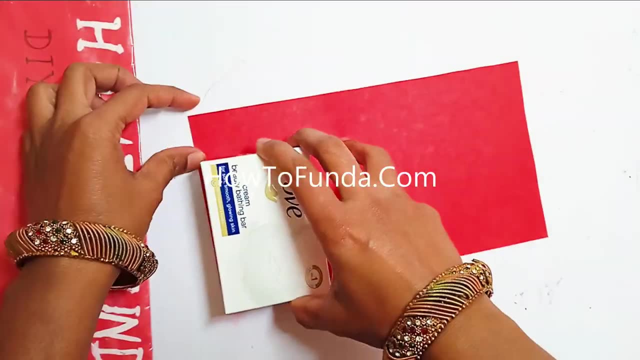 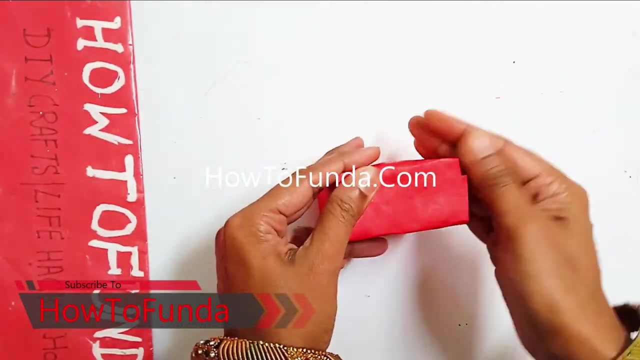 I can hear the demons call when they do what they do, And now I feel like taking off. find a place with a view. The pain is never gonna stop if it's controlling you. I know the time can heal it all. I just gotta get through. 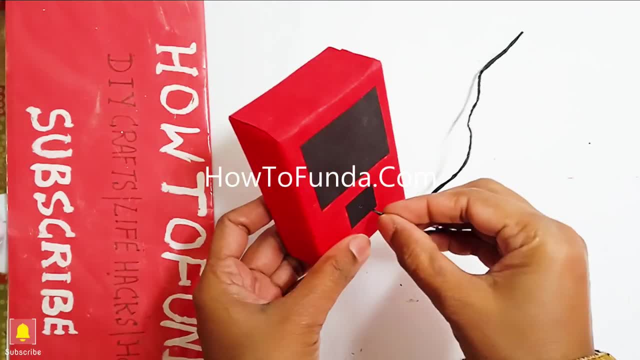 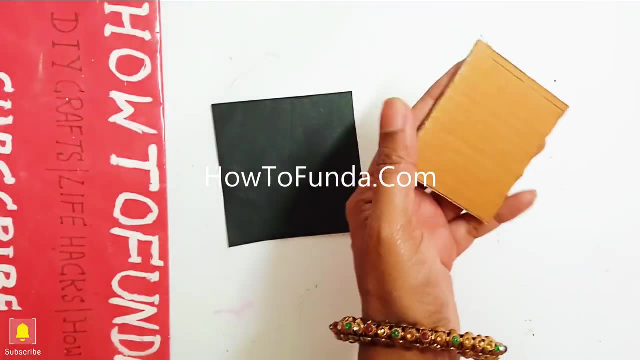 I just gotta get through. I just gotta get through Cause I feel like taking off. find a place with a view. The pain is never gonna stop if it's controlling you. I know the time can heal it all. I just gotta get through. Sometimes I feel like all is lost, but I know it's not true. 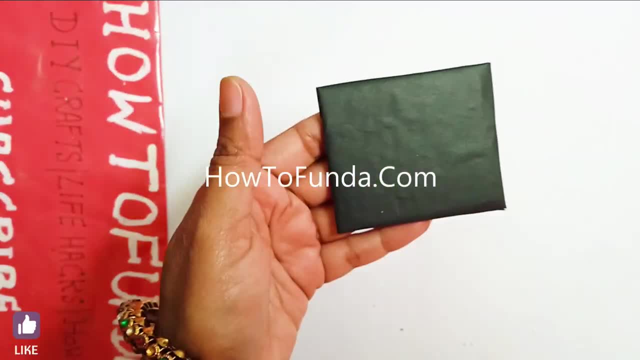 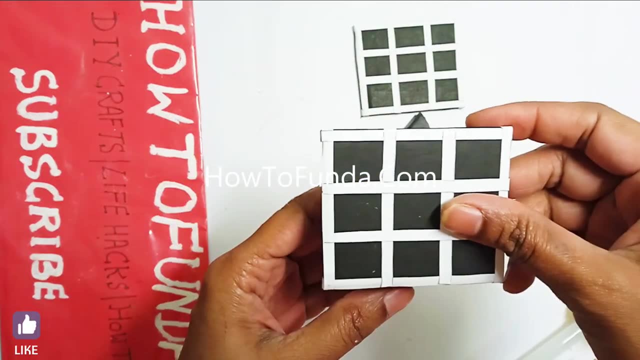 I wanna put up all my walls cause I'm not in the mood, But then I cut myself off from the rest of the room. I know the time can heal it all. if you're patient and soon, It can all be worth it all the searching. 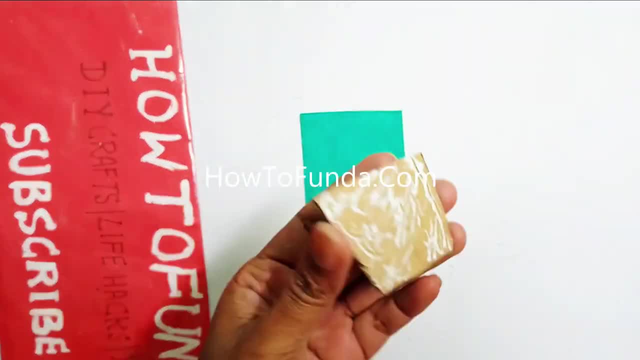 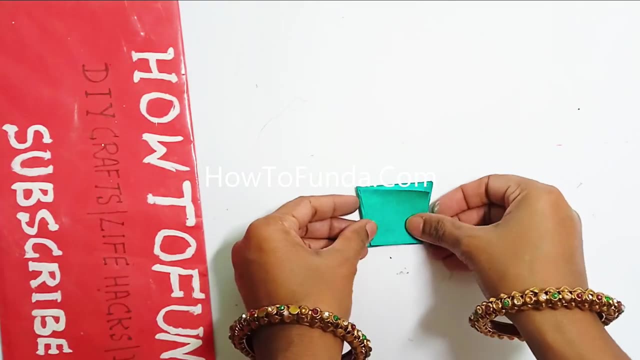 Pain is never really permanent, but damn, it hurts man. I can feel all of the turbulence and it's concerning. I've been searching for a purpose. I hope it's worth it. This society is really trying me, Ain't no hide and seek, I hide to be far from anxiety. 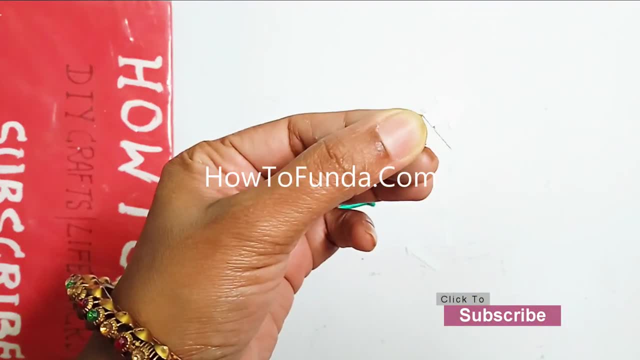 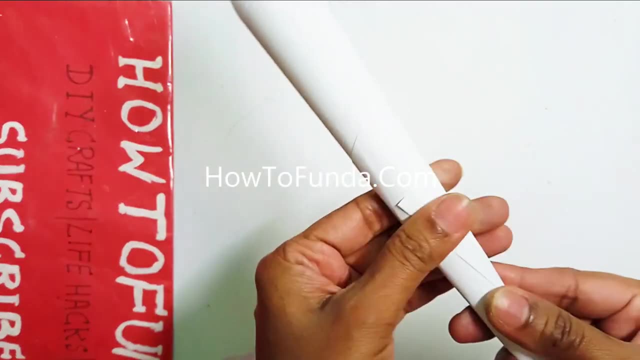 I need my space. I need my privacy. I need some silence, please. you're all too loud. You don't speak quietly. opinions violently Thrown across every surface. it makes me nervous. It's the world honestly burning. that's all I'm learning. 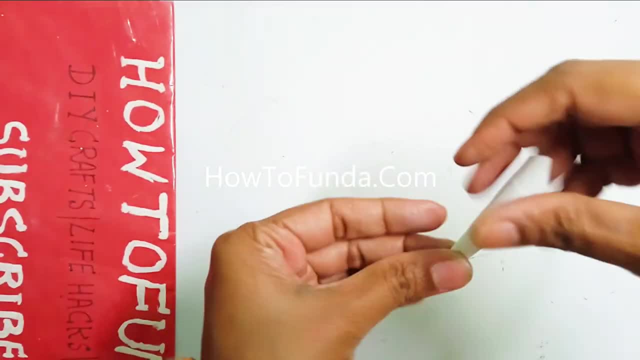 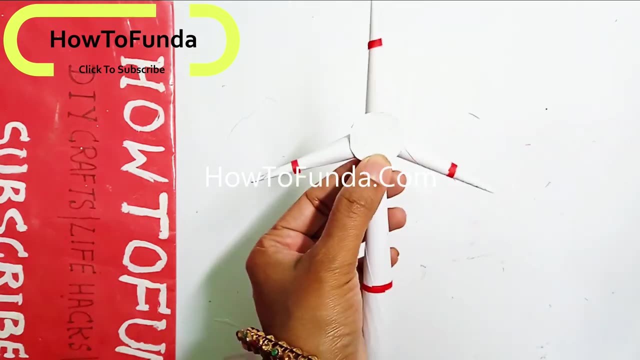 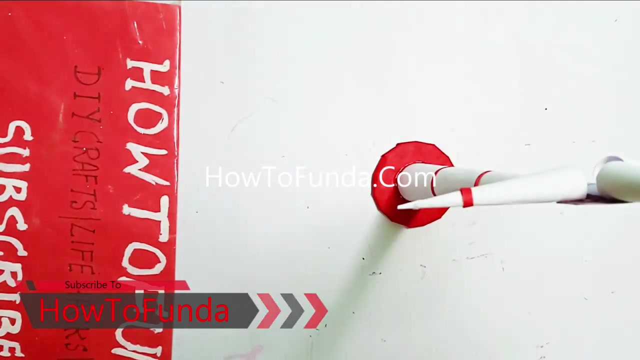 Hope that we can make a turn and start reversing. All our minds have put their minds to work. All our minds have put their minds to work And we got some work. man, I just gotta get through, gotta get through. I just gotta get through, gotta get through. 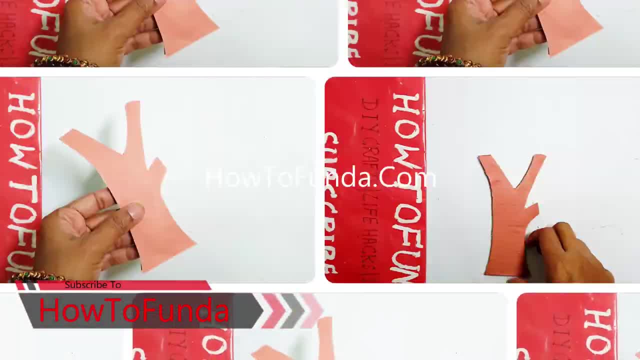 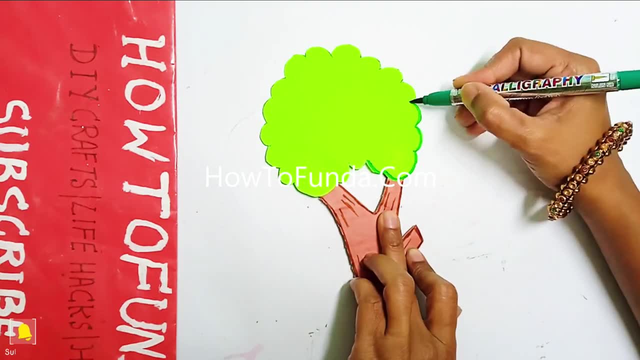 I can hear the demons call when they do what they do, And now I feel like taking off. find a place with a view. The pain is never gonna stop if it's controlling you. I know the time can heal it all. I just gotta get through. 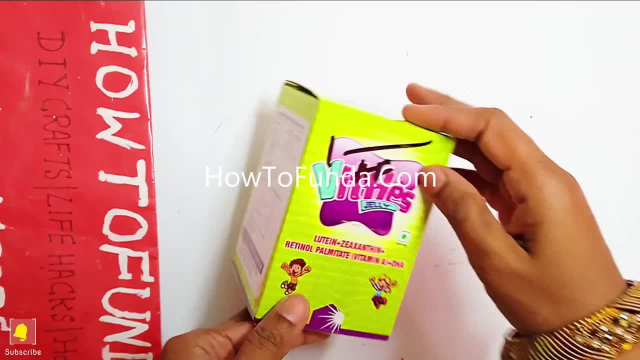 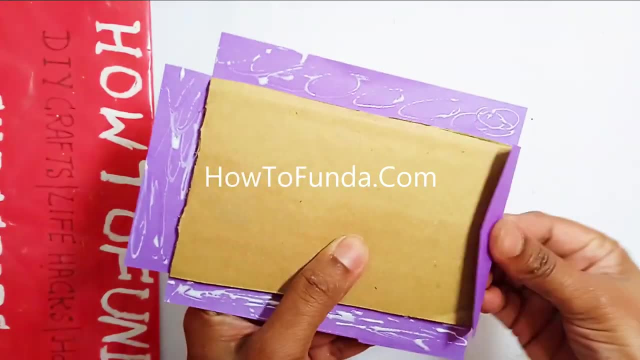 I just gotta get through. I just gotta get through, Cause I feel like taking off. find a place with a view. The pain is never gonna stop if it's controlling you. I know the time can heal it all. I just gotta get through. I just gotta get through. 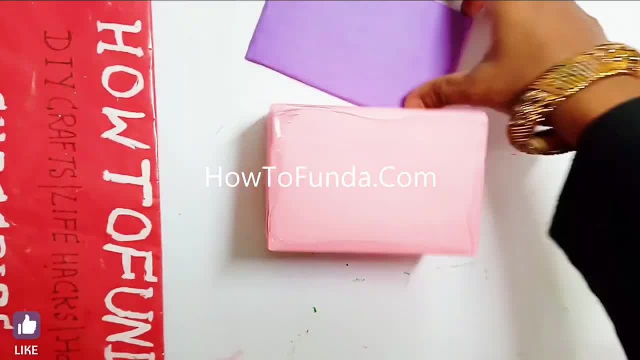 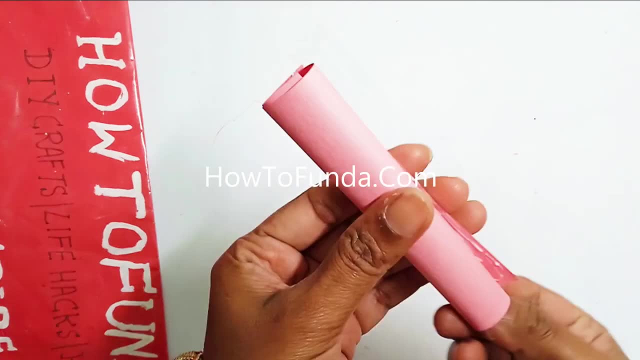 Gotta get through. this life is a nuisance, tie-ups and loosens. I try to be human, find a solution. my evolution, A place like this. it didn't exist. we made it like this, So you can go pick the bad or the good. got a glass half-wish. 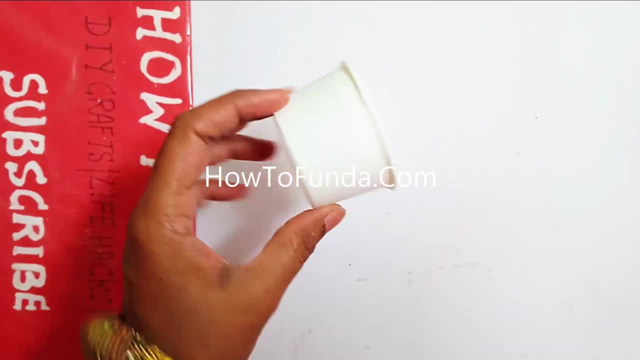 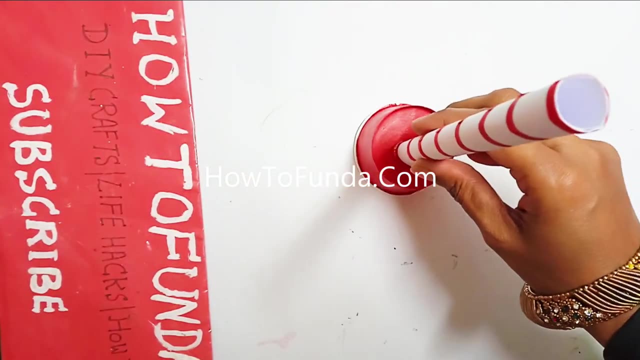 I know it's easier to hide than just to lay low. Not everyone can see, but I know And life has got a halo. I'm standing in the red inside a payphone Just wanna break. no, I'm not gonna give in. take a last shot. 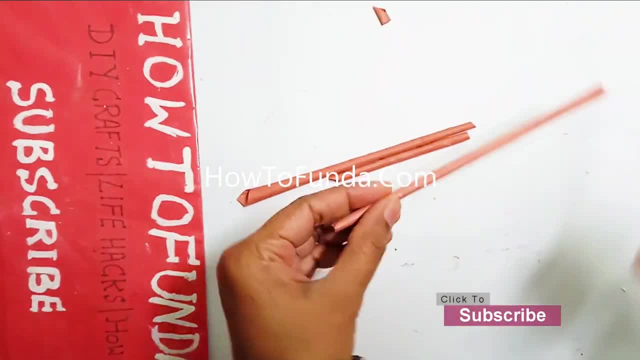 Michael J Wynn. no, I'm not a robot. I'm in my own skin. Never get lost when thoughts pull you in. I miss the old you. we died with a purpose. All the energy around me felt nervous, Scared. I would pop out fast to the surface. 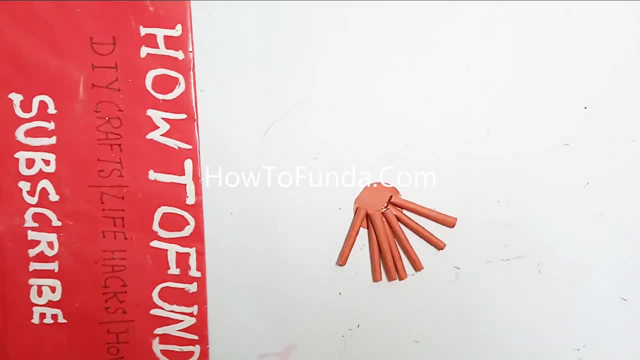 Had to cut it off before you made me worthless, Torn apart, I've been torn and scarred. I had a given heart, but now I'm freaking smart. I'm keeping up my guard. I'm hiding every card, A royal flush of love. you never know what's hard. 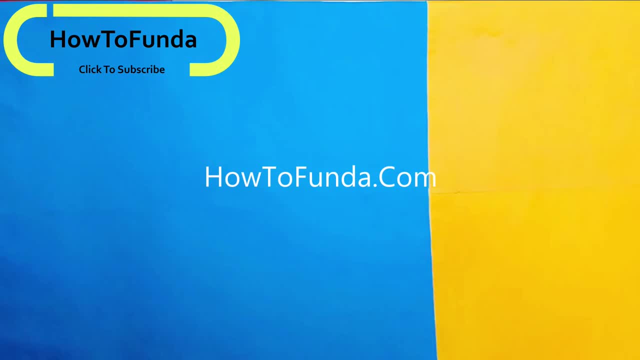 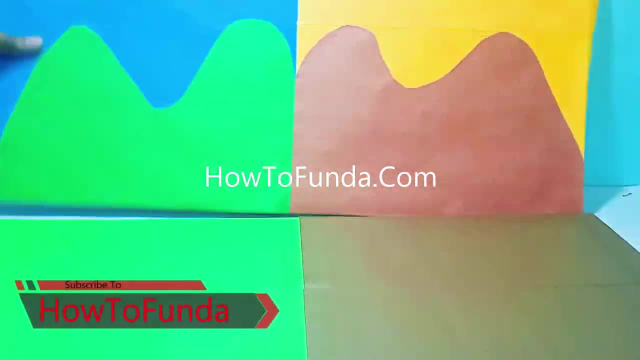 With a back to the mat gonna see where I'm at. I'ma fight like I'm mad. I'ma be something that Be me. nice try, but they'll see I achieve everything While they stay salty. I just gotta get through. gotta get through. 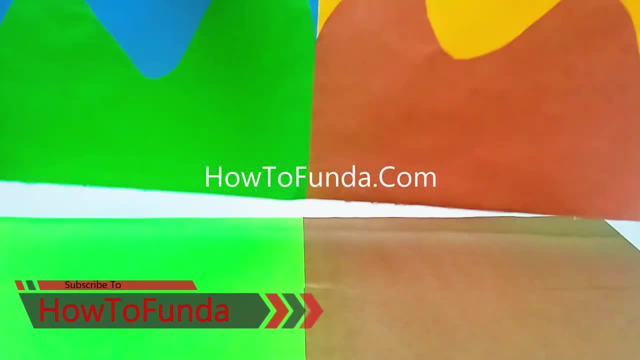 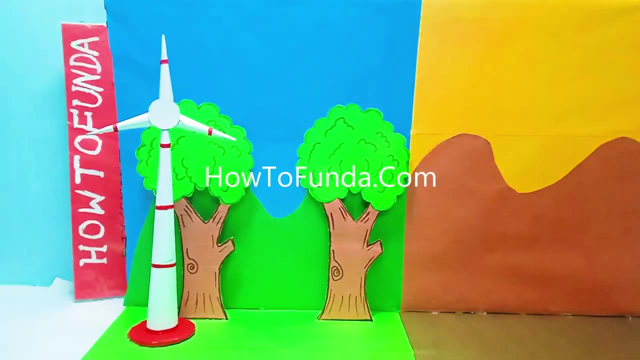 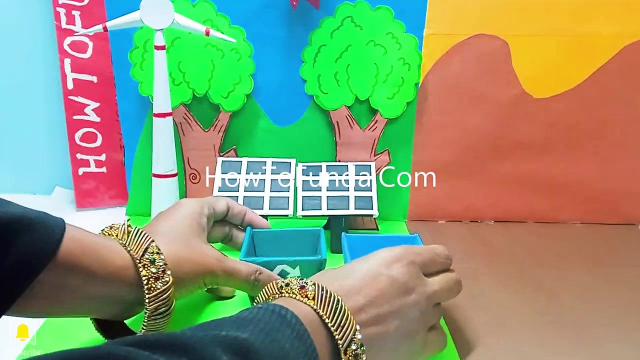 I just gotta get through. gotta get through. I can hear the demons call when they do what they do And now I feel like taking off, find a place with a view. The pain is never gonna stop if it's controlling you. I know the time can heal it all. I just gotta get through. 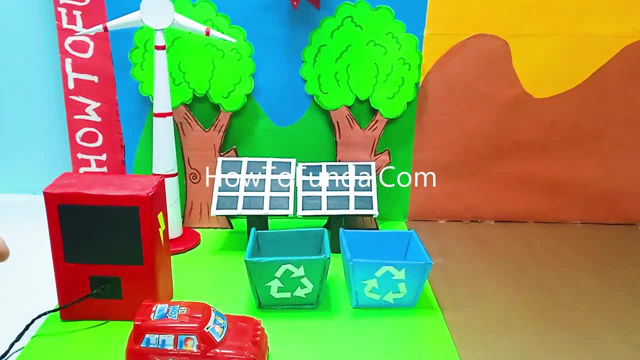 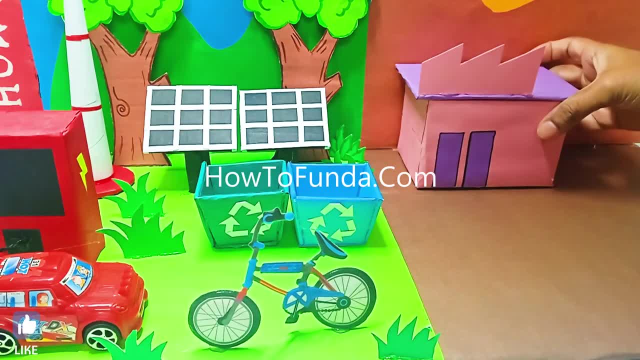 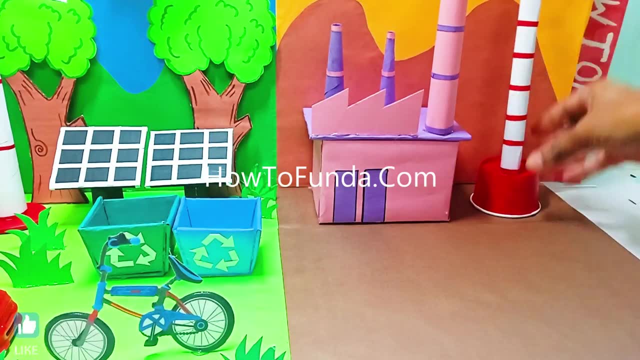 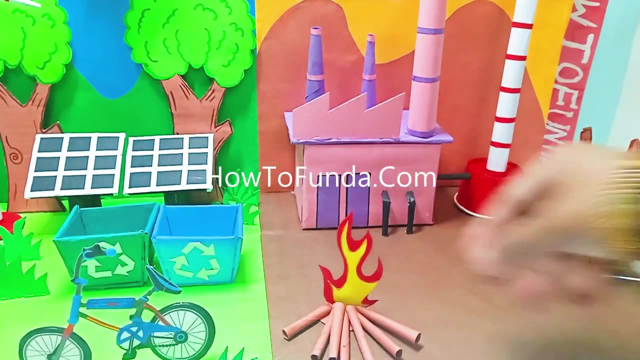 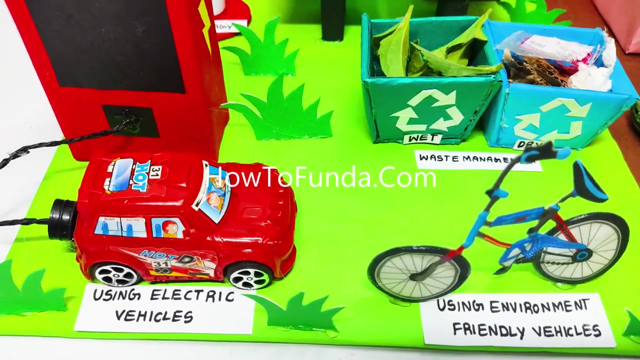 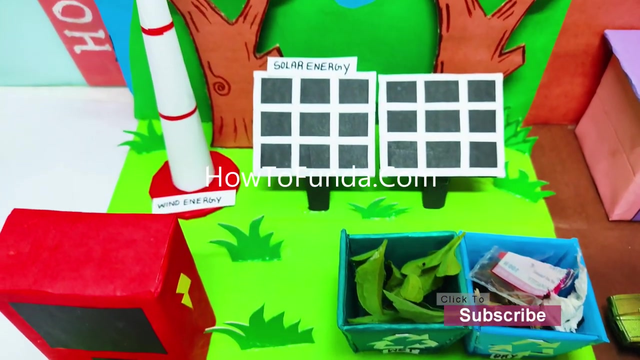 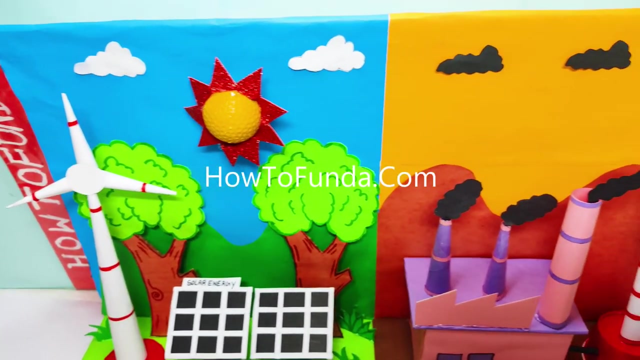 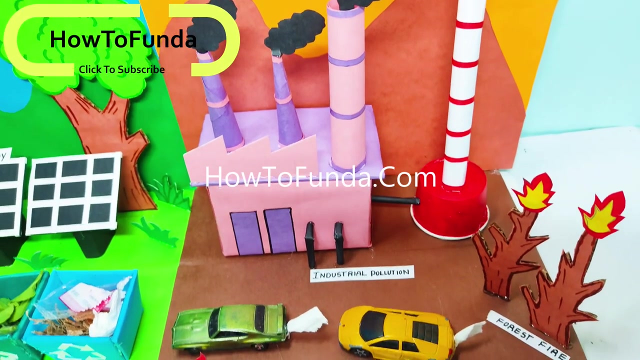